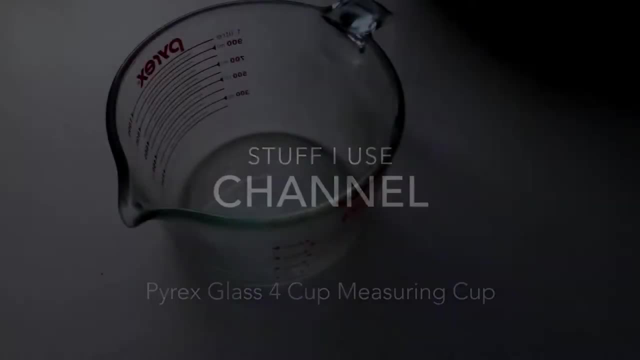 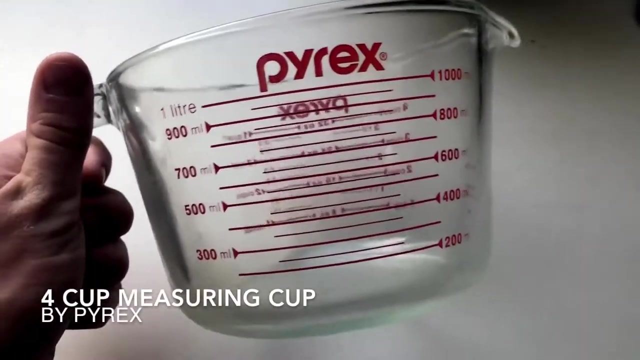 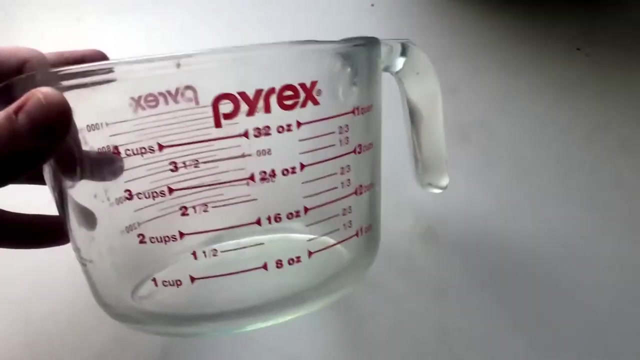 All right, y'all. What's going on today? Today I'm going to be talking to you guys about the Pyrex 4-cup measuring cup. We're on the leader's hut- 4-cup measuring cup. Yeah, Pyrex is great. I mean, if you know anything about cookware, Pyrex has been around for. 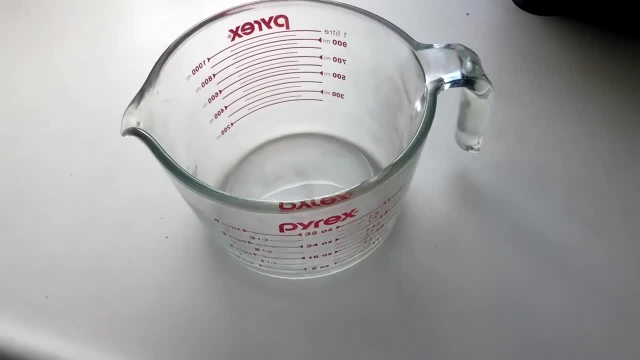 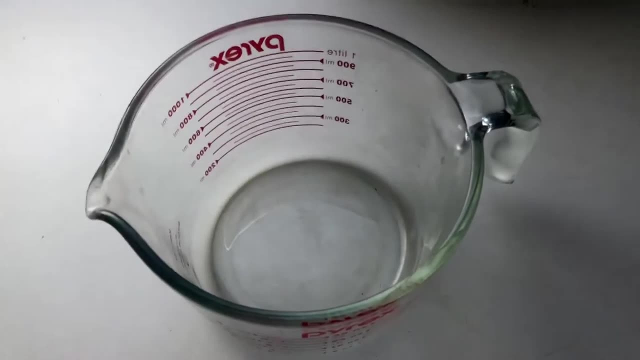 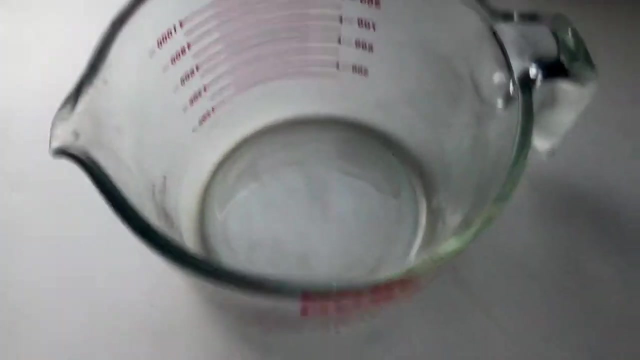 Jesus, probably over a century now They've been making, you know, everything from measuring cups to storage containers and beyond, Really everything for prepping kitchen, good prep cookware, things like that. They're just a very, very well-rounded company. They are a very strong. 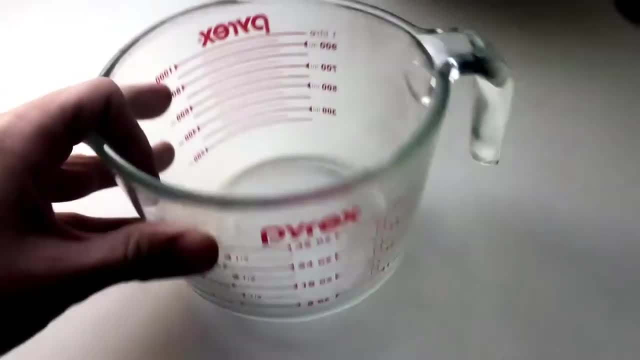 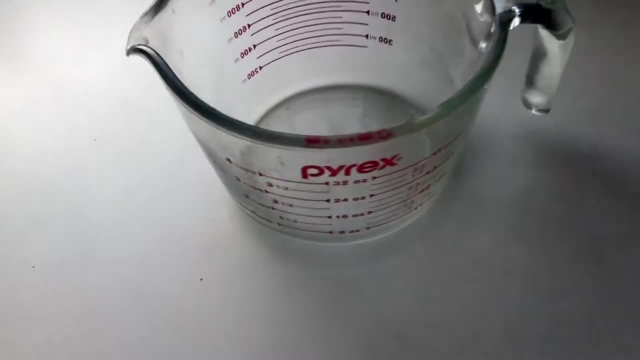 brand. I guess you could say and just make great, ultra-recognizable cookware Right off the bat. you can tell it's them just because you know you have that bright red and Pyrex is kind of known for that. There are some companies that have definitely taken it from them and tried to do it. 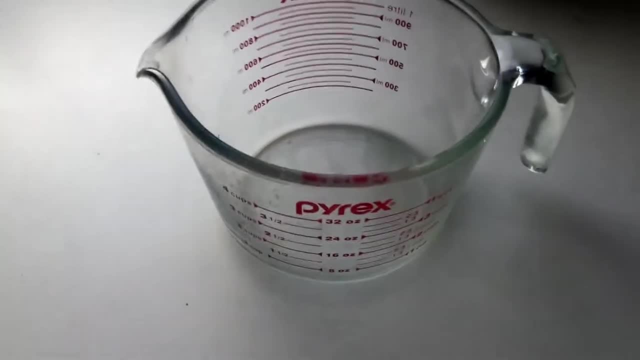 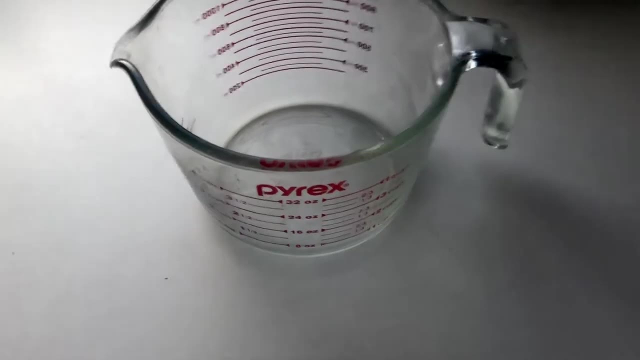 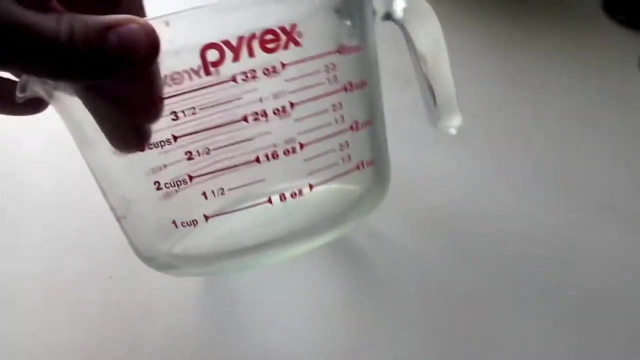 but they are. They are the best by far, in my opinion. What I love about these Pyrex cups is that they are very, very easy to read- Very easy measuring cups to read. That's thanks to the bright red letters that are on them And it's maybe a little bit harder to tell, but these are definitely a. 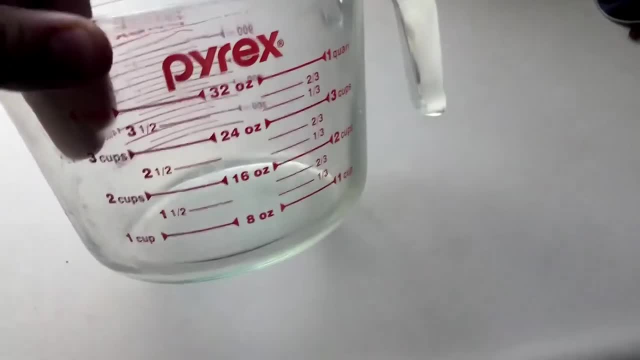 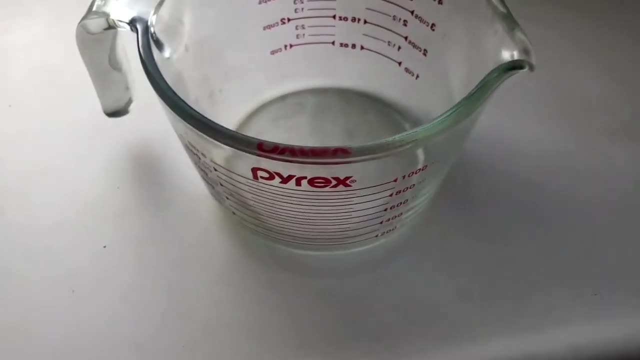 brighter than darker red. So you know, whatever liquid you're putting in there, most likely you'll be able to read this very, very easily. There's only some liquid that I could think of that might be a little bit difficult, like tomato juice, but you know. 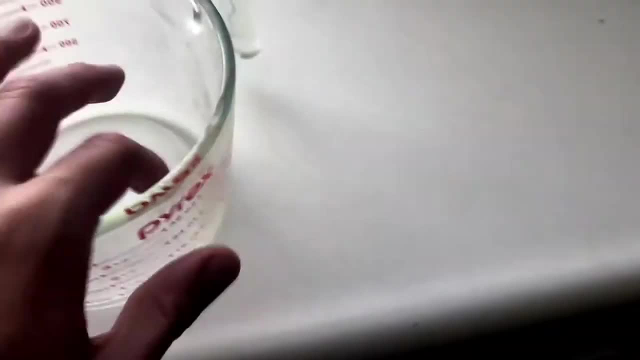 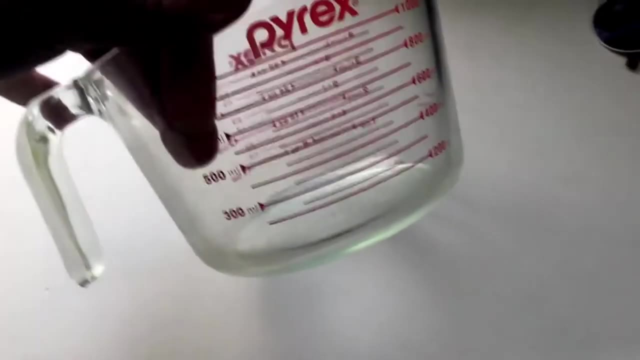 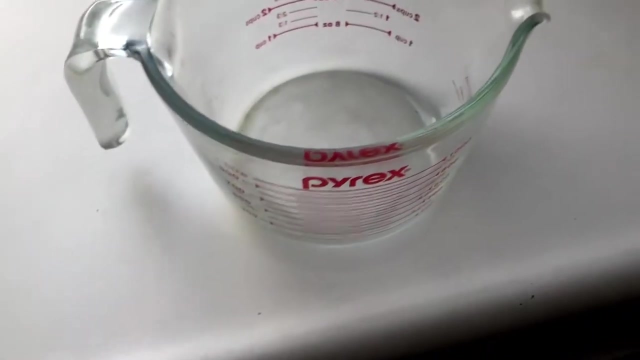 that's. that's that You also have the four cup and ounce side as well as the liter and milliliter side over here. So depending on the recipe there you know you don't have to convert. It's nice that they basically gave you both to work with. 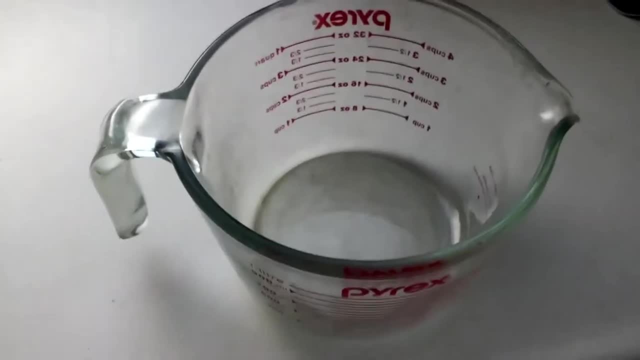 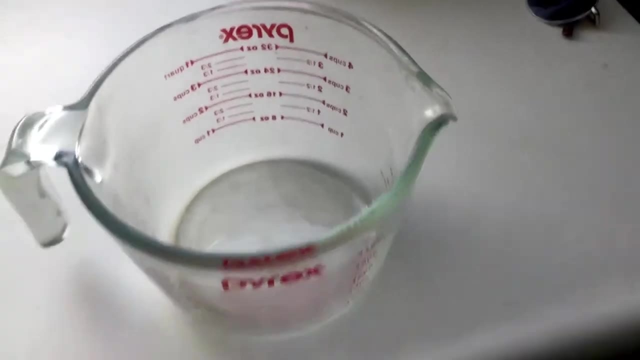 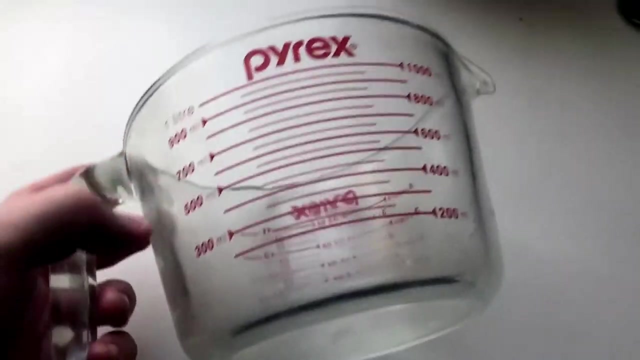 Also just makes sense because this makes it an international product as well. so it's probably best that they did that anyway. The lettering on here, Leslie, is very, very bold and very clear. You know they weren't trying to go for like a minimalist design or anything, It's straight up. you know, practical and 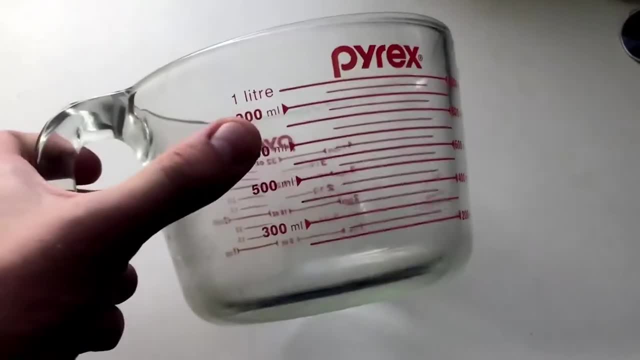 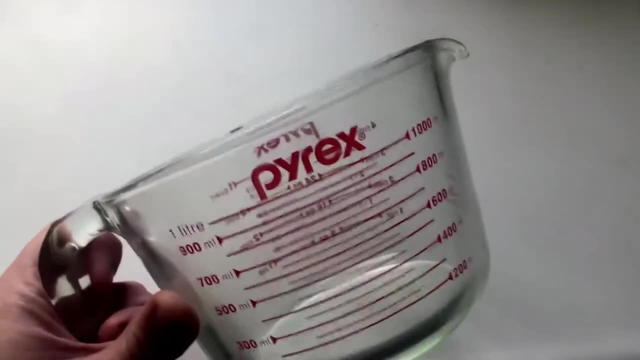 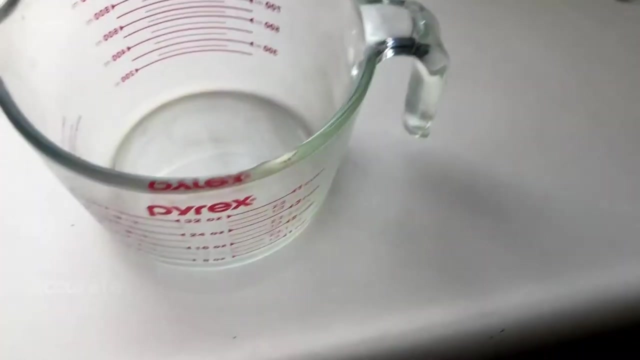 efficient the way that they they did the numbers on here. It essentially looks like, you know, some big red, clear sticker with bold font and very, very accurate as well, Which is important for a measuring cup, I mean that's you know. it should work in that way. It should be very, very. 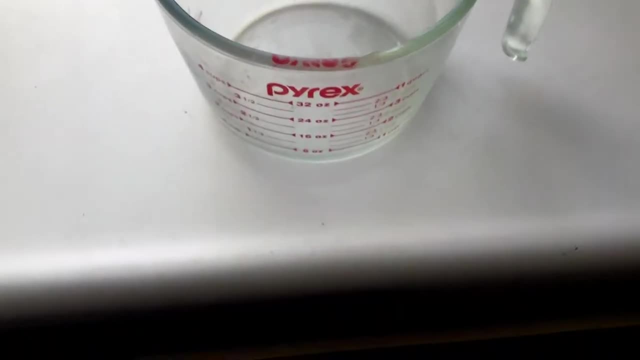 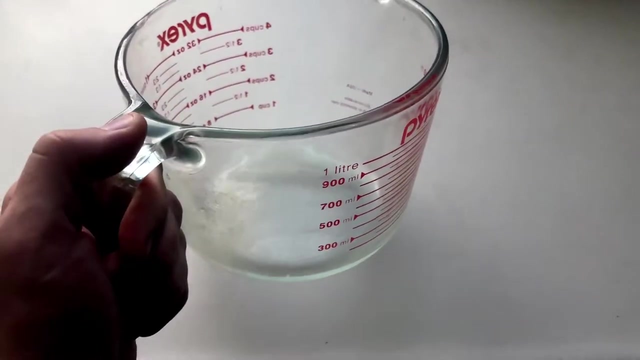 accurate, and it is. The handle is very comfortable as well on this thing. It gives you enough room. It's pretty far out. Also have this little indent which you can kind of see at the top. It's perfect for your thumb, Kind of gives you. 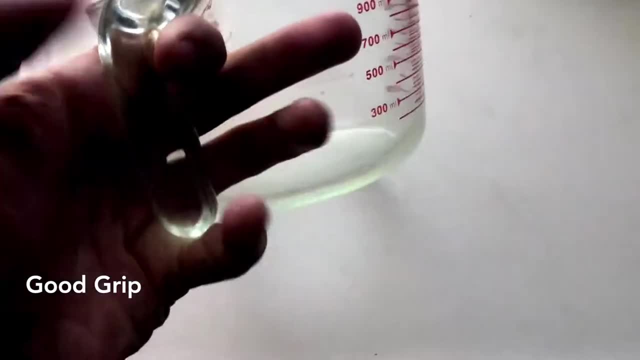 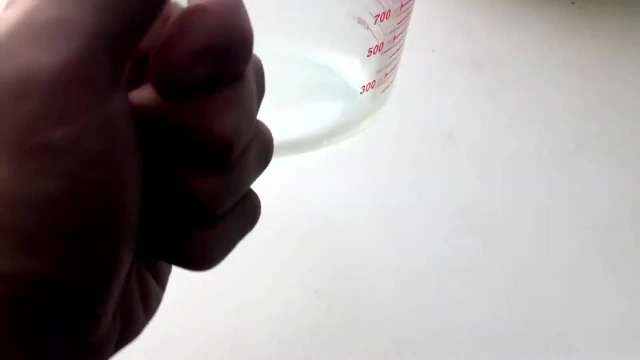 like an ergonomic way to grip it. I wish maybe it was a little longer at the bottom, although it would maybe touch, but I don't know. it just seems like sometimes, like it doesn't even go all the way to the end of end of my hand And it's already kind of heavy right now. So when you do have liquid in, 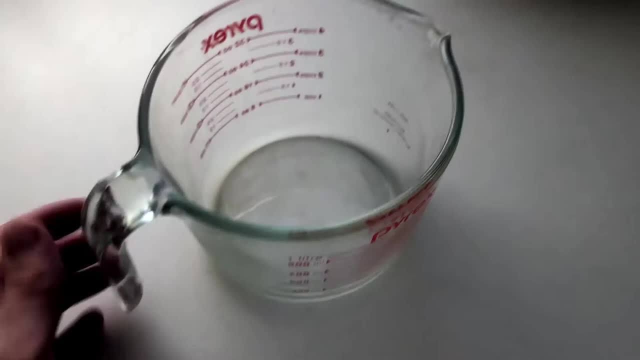 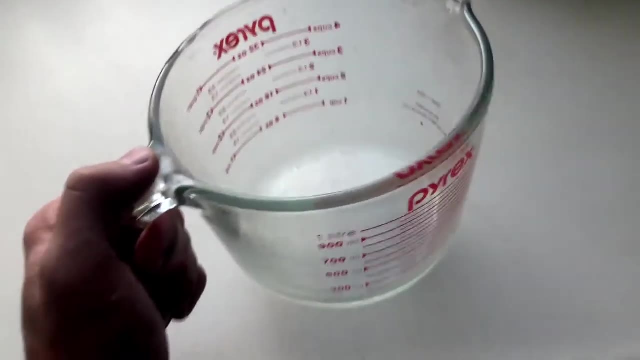 here can get even heavier. And the issue is, when you have hot liquids you have to hold it with a towel and try and pour it. So that's maybe one thing. I have a design change, A design flaw, I guess maybe you could call it, But uh, not the. 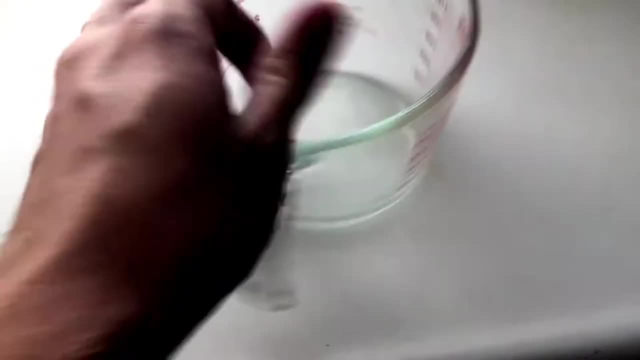 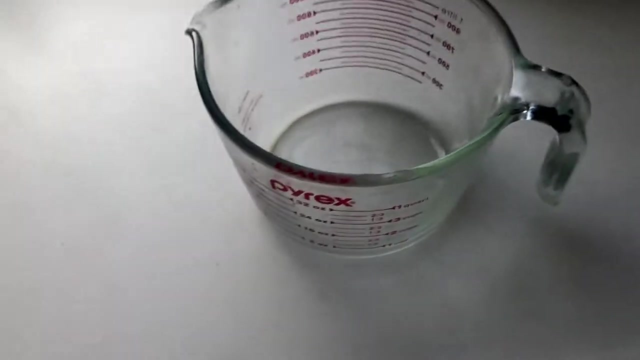 biggest deal in the world. The glass on here is totally non-porous, Very, very, very tough glass. It stays odor free. It stays stain free. Again, I've had these a this, this Pyrex cup, for a very long time, as well as my other ones. They haven't. 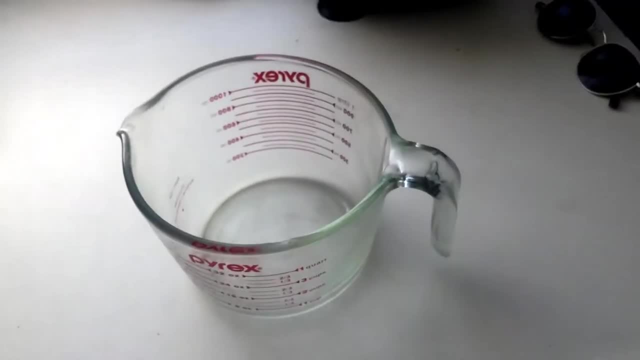 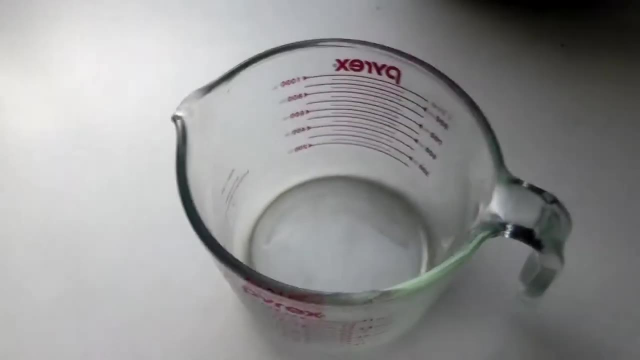 retained any sort of stains, I mean sort of odors or anything gross like that. So you know. you know that after every wash you have one that's pretty much as good as new, you know, And then ready to roll for your next cooking adventure. They are. 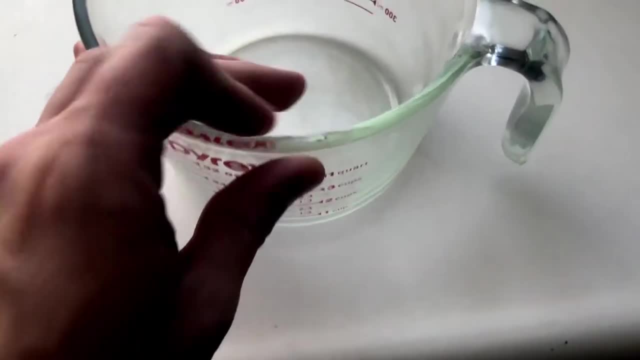 very durable as well. I've definitely dropped this multiple times. The one time that I dropped it from the highest point, I got this little. you can kind of see there's a chip right there. That was the most that I got from it, from dropping it. 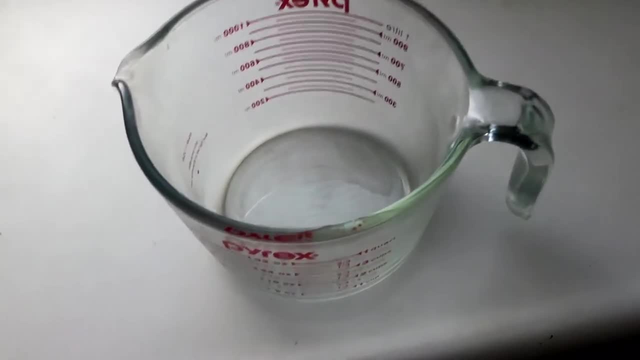 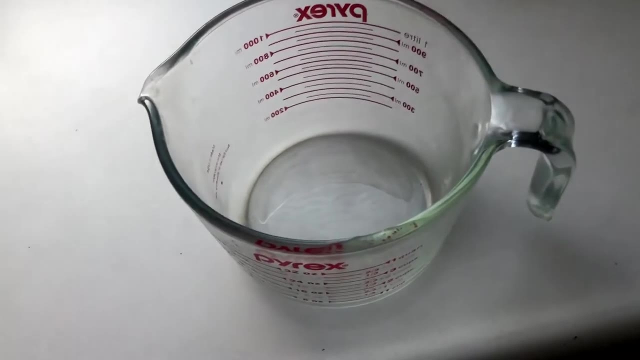 on a tile floor. So very seriously durable glass, Very thick too, Makes it great for, you know, a lot of different uses, One of those being that it's microwavable safe. You know, obviously don't want to nuke this thing to death.